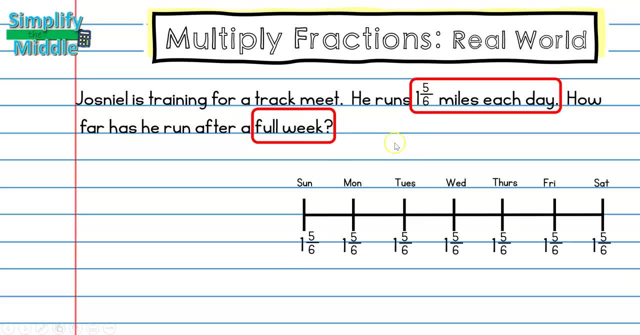 six miles. This is going to help me create an estimate. I can see I have seven days and I can see that I have one in five, six for each of those days. So I'm gonna round this to two. So my estimate is two times seven is 14.. Now let's go ahead and multiply. 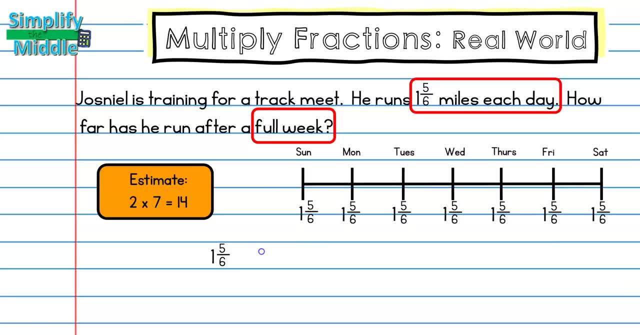 and see how close I was to my estimate. If I'm not close, then it means that my answer is not reasonable and I probably did something wrong. One in five sixths is going to convert to 11 sixths, So I'm gonna divide it over the denominator of one. Looking across, I don't have any common factors. 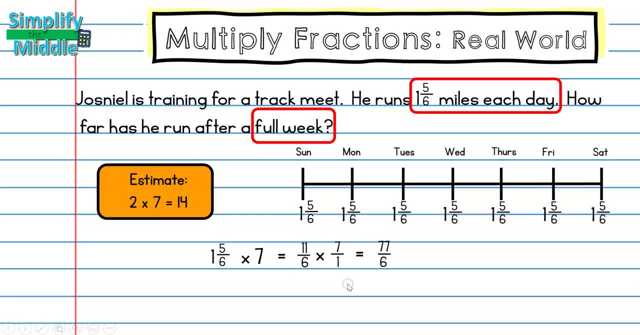 so I'll just multiply straight across and I get 77 sixths. And if I divided 77 by six I end up with 12 and five sixths. That's pretty close to my estimate of 14.. So I think my answer. 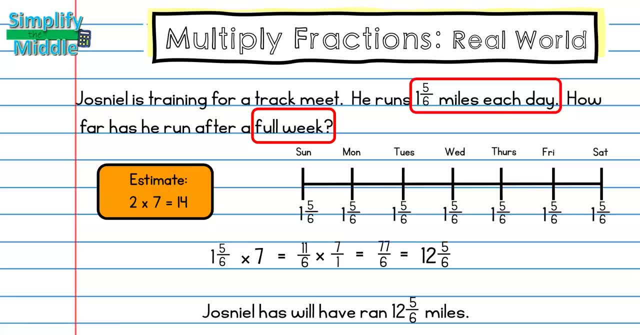 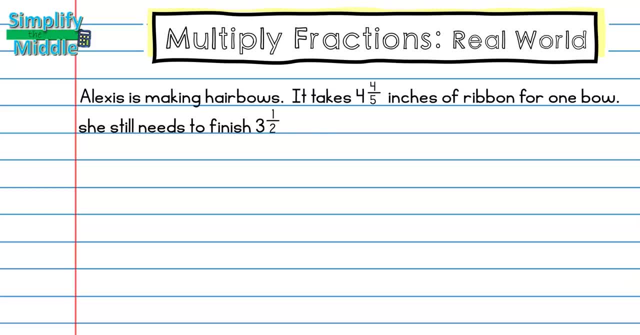 makes sense. Joe Sneel will have run 12 and five sixths miles. Our next problem, Alexis, is making hair bows. It takes four and four fifths inches of ribbon for one bow. She still needs to finish three and a half more. How much ribbon will she need? 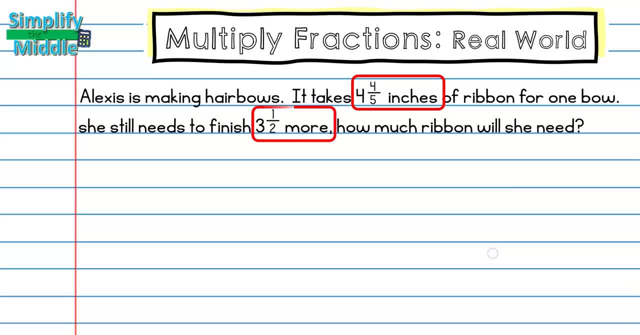 Well, I know that it takes four and four fifths inches for one and that she's needing three and a half more. So this problem didn't give me any clue words either, but I can tell that I'm going to be repeating four and four fifths, three and a half more times, So I'm going to use a number line. 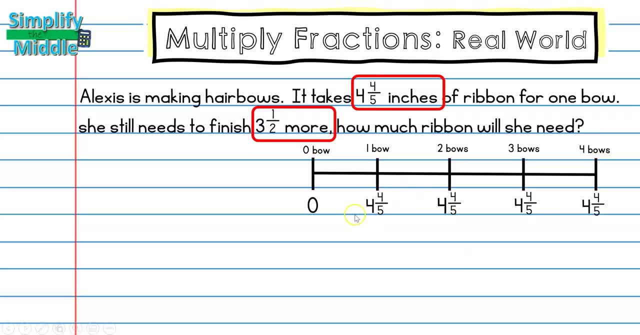 a little differently This time. I know that each bow is four and four fifths, So I'm just going to go ahead and do my number line where I am jumping from zero to one bow, two bows, three bows and three and a half. 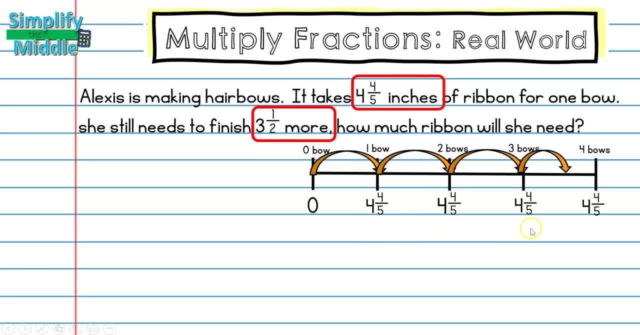 Because this is really close to five. I know that she's in between three sets of five and four sets of five, So my estimate here is going to be between 15 and 20.. So I get an estimate of 18.. Let's go ahead and multiply and see how close I am to that estimate. 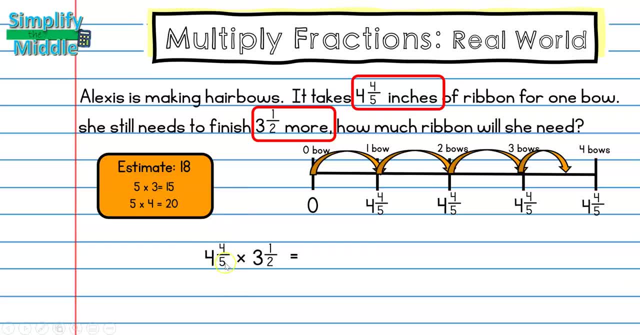 I know four and four fifths converts to five times four is 20 plus four is 24 fifths. Two times three is six plus one is seven, seven halves. And I can see I have a common factor between 24 and two. So I'll cross cancel and divide 24 by two and get 12.. Divide two by two. 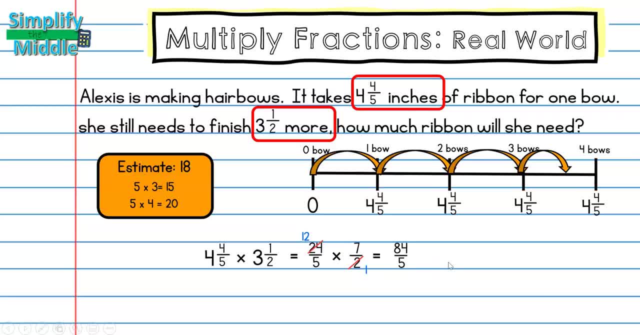 and get one. So my answer is 84 fifths. I will need to divide to find that I have 16 and four fifths For my answer. So Alexis will need 16 and four fifths inches of ribbon, And that's pretty close. 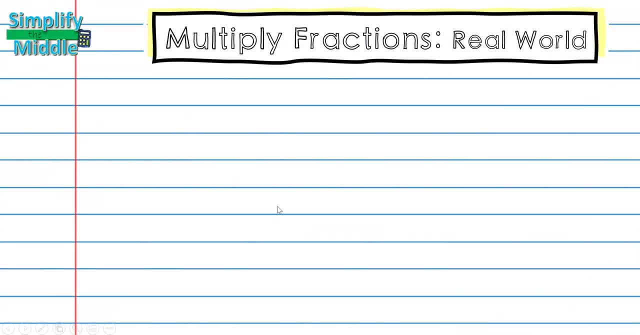 to my estimate of 18.. So my answer is reasonable. For my next problem, there is nine tenths of a kilogram bag of bird seed left. You use two thirds of what's remaining to fill your bird feeder to the top from empty. How much seed does your bird feeder hold? I know nine tenths of a kilogram is. 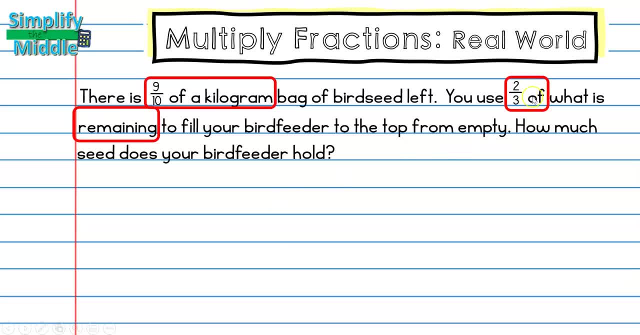 important information, And this time I did use a clue word Of, so I have two thirds of it remaining. I'm going to draw out my nine tenths And then I am going to cut that into two thirds. So if I can look here, I can see that all of these parts are representing. 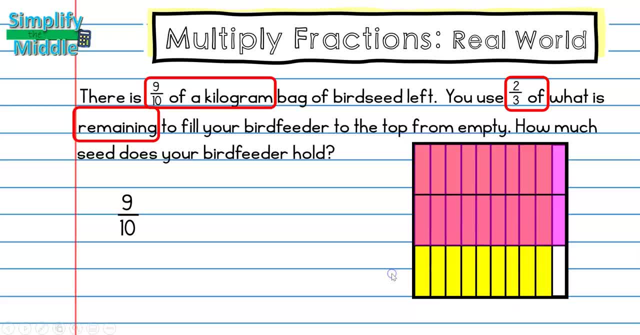 the answer, And then this is representing the denominator for my answer. So I'm just going to multiply nine tenths times two thirds. I'm going to cross cancel here because I see they both share a common factor of three. So nine divided by three is three, and three divided by three is one. Cross cancel here. Two divided by. 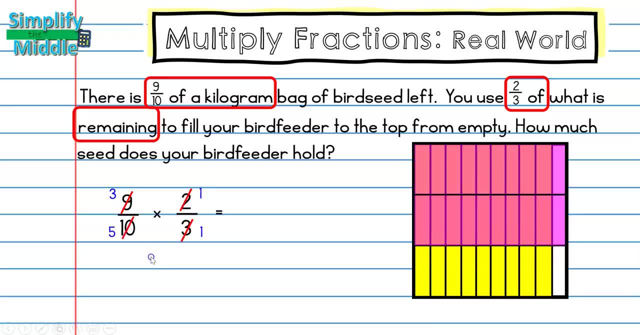 two is one and ten divided by two is five, And I end up with an answer of three fifths. If I was to multiply straight across, I have 18 thirtieths and that's going to reduce to three fifths, So that 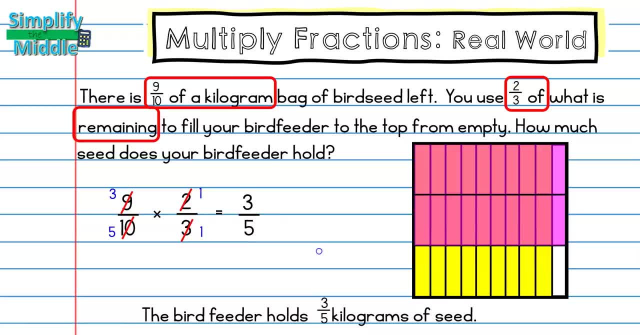 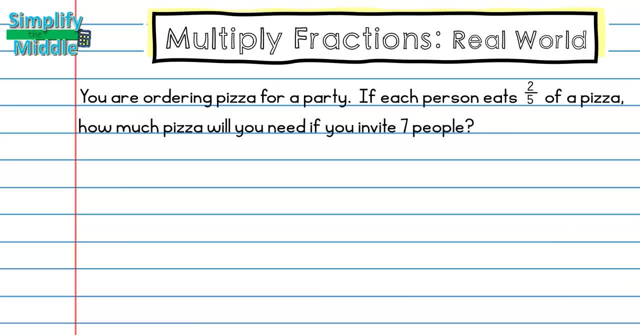 makes sense. So the bird feeder holds three fifths kilograms of seed. For my last problem: you're ordering a pizza for a party. If each person eats two fifths of a pizza, how much pizza will you need if you invite seven people? This problem has a couple of